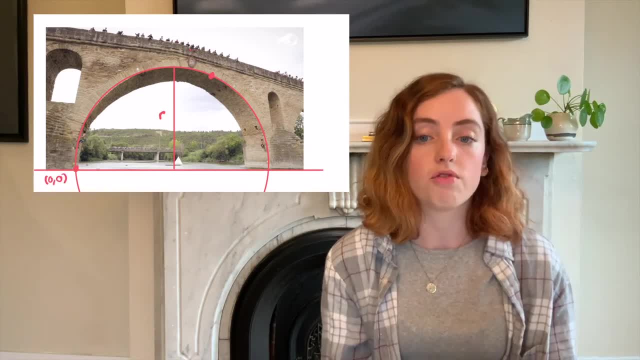 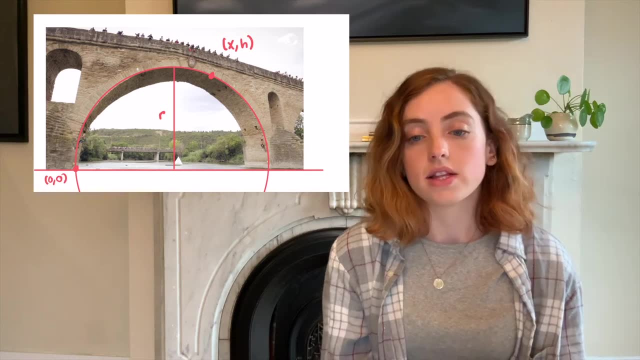 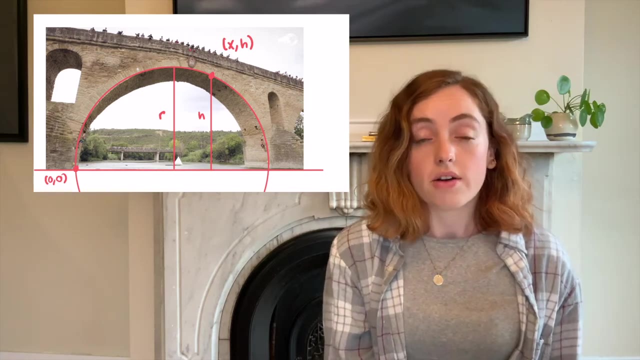 Next I'm going to mark the point where Rustem Gelmanov falls in his climb. The coordinates of this point will be called x, h. So in this situation, h is the height that he climbed to before he fell. First I'm going to calculate this quantity, h. 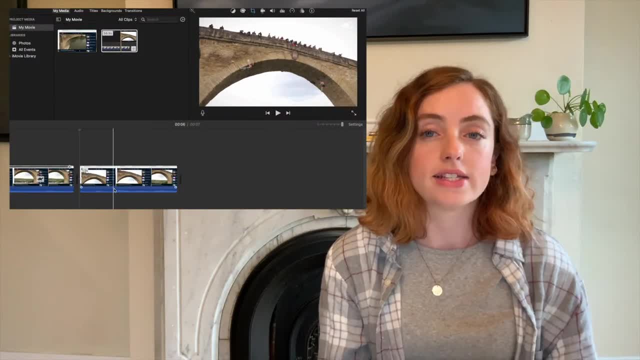 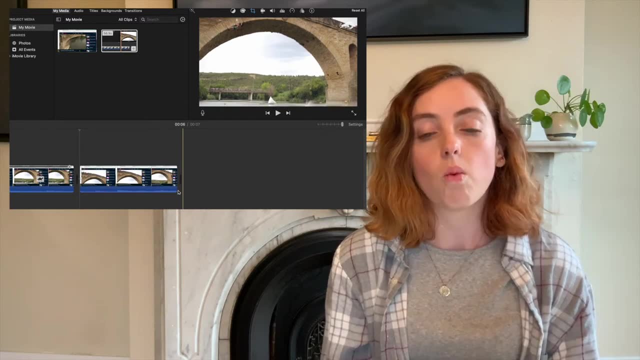 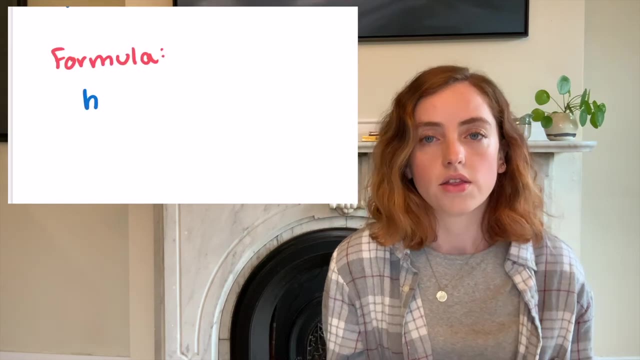 By analyzing the footage from when his hand left the wall to when his body was fully submerged in water, we can see that his fall took about 1.3 seconds. His acceleration is approximately 10 meters per second squared. There is a formula for the total height of his fall in terms of the time. 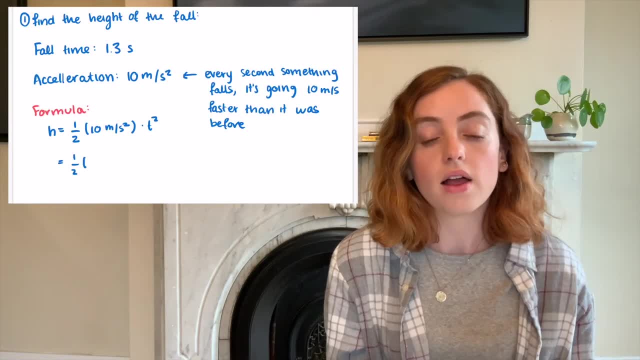 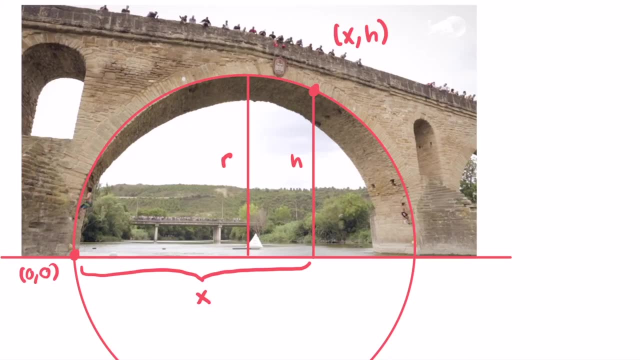 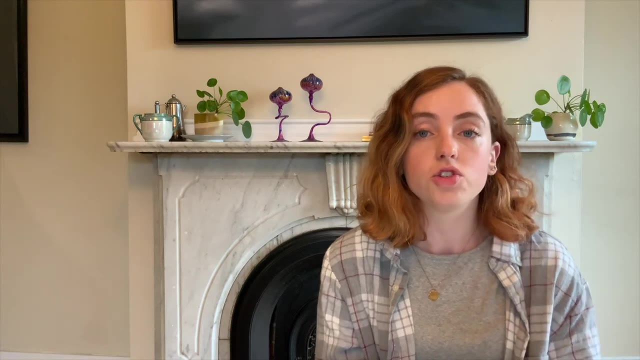 In total, this tells us that he fell approximately 8.45 meters, or 27 meters. So this is the quantity h in our diagram. Now I'm going to estimate the radius of the bridge arch by zooming in a bit on this footage. 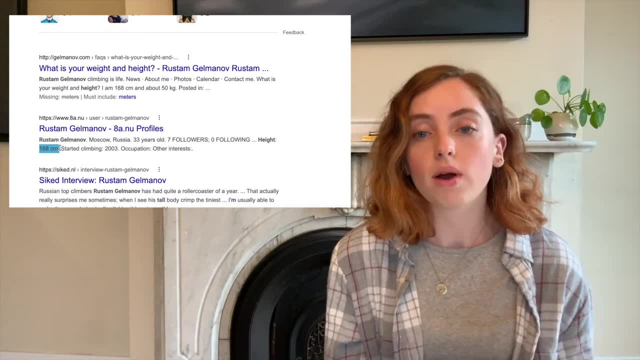 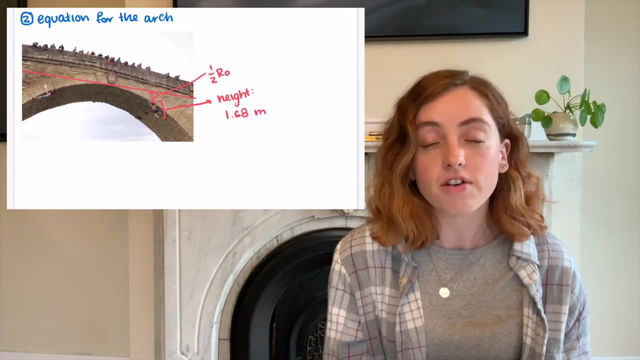 Rustem Gelmanov is a height of 1.68 meters. To me it looks like the distance from his hand to the top of the arch is about half of the length of his height, So that gives us an additional 0.84 meters. 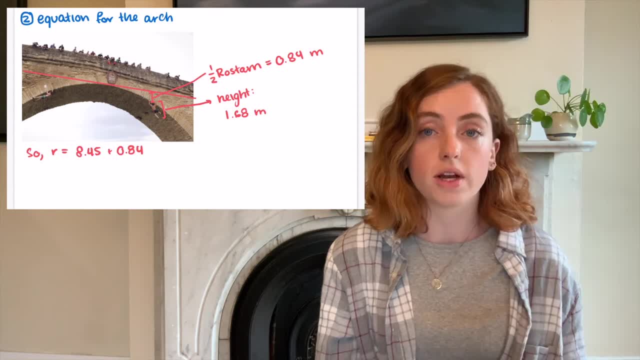 In total, this tells us that the radius of the arch is about half of the length of his height. So that gives us an additional 0.84 meters. So that gives us an additional 0.84 meters. So that gives us the radius of the bridge arch is the height h that we already found, plus 0.84 meters. 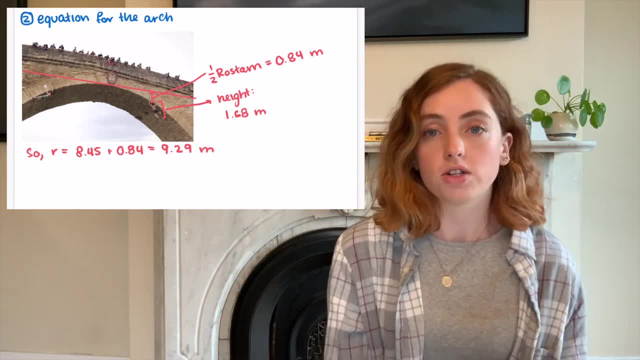 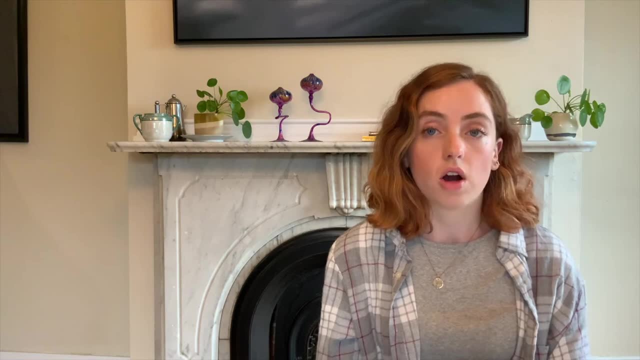 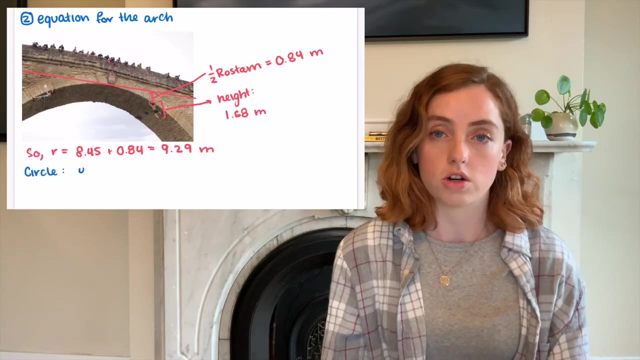 So this gives us the radius of 9.29 meters, which is approximately 30.5 feet. Now we can write down an equation for the arch of the bridge. I'm going to start with the equation for a circle which is: y² plus x² equals r², where r is the radius. 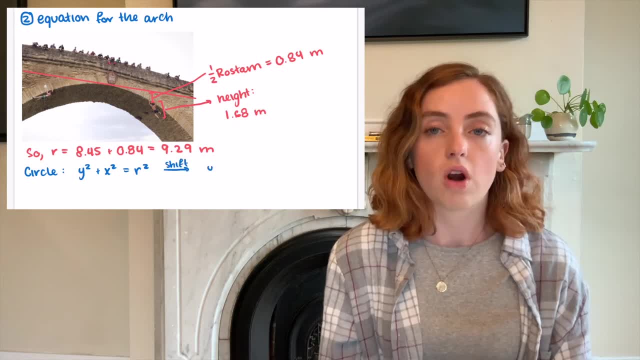 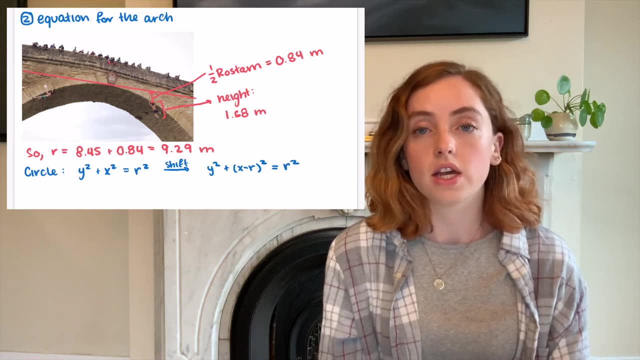 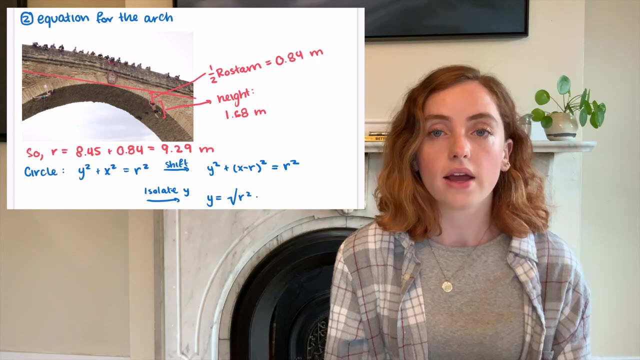 We can shift this to the right by subtracting our test further, So it becomes Xni pleased. subtracting r from x, So we get y squared plus x minus r squared is equal to r squared. From this we'll move the x part to the right side of the formula, isolating y, and then take the square. 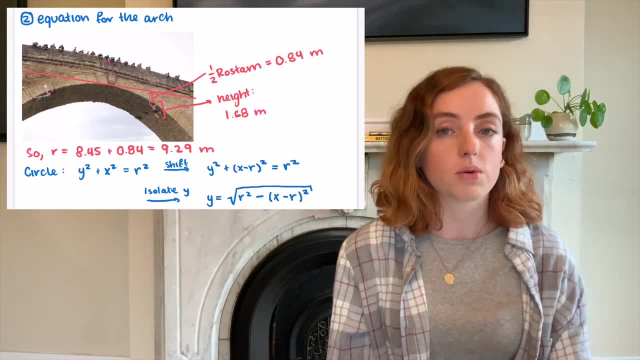 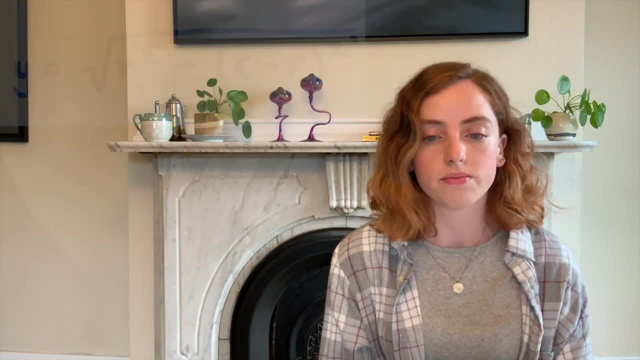 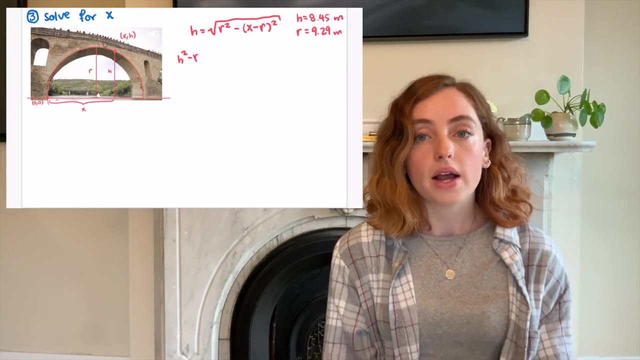 root. In this scenario, we want to take the positive square root so that we get a semicircle in the upper half plane. This gives us the following bridge equation: Now I want to solve for x the location of Rustam Galmanov when he fell, So I'm going to plug in h for y, since h is. 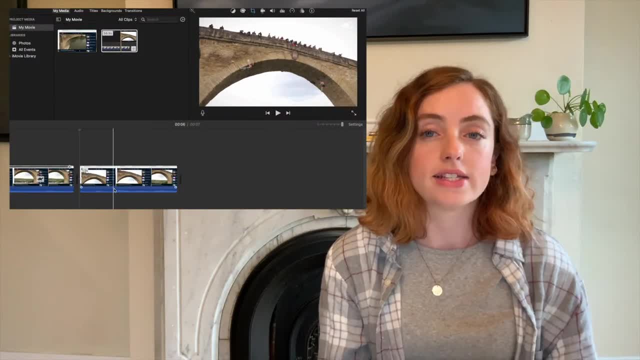 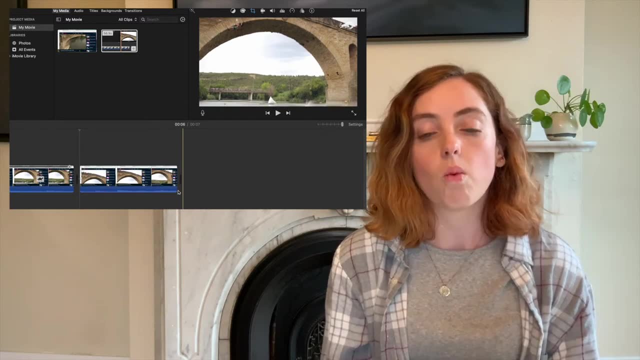 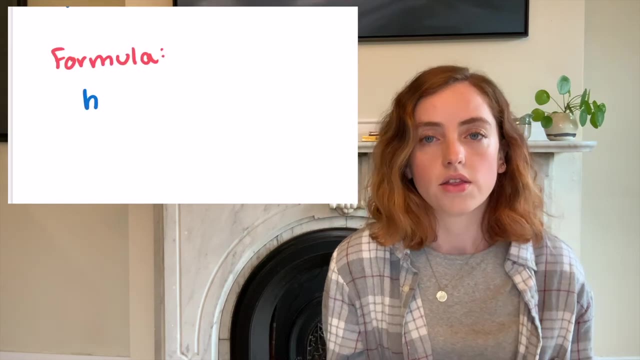 By analyzing the footage from when his hand left the wall to when his body was fully submerged in water, we can see that his fall took about 1.3 seconds. His acceleration is approximately 10 meters per second squared. There is a formula for the total height of his fall in terms of the time. 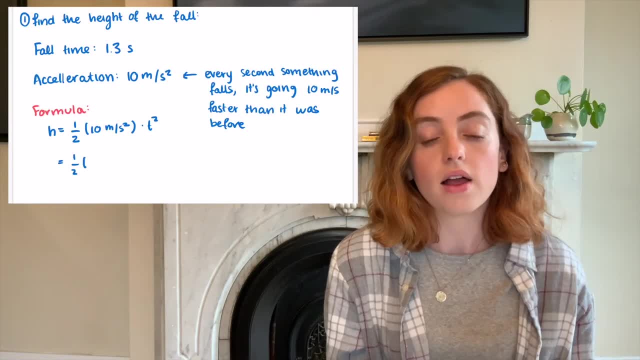 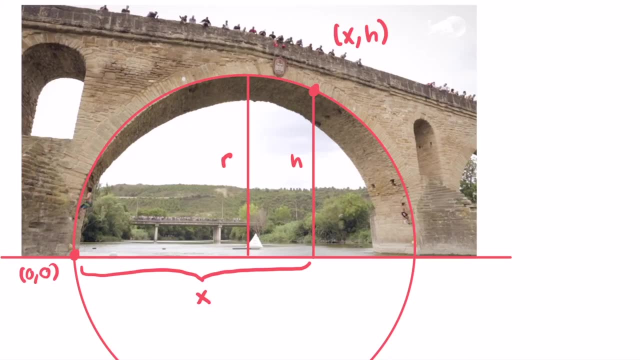 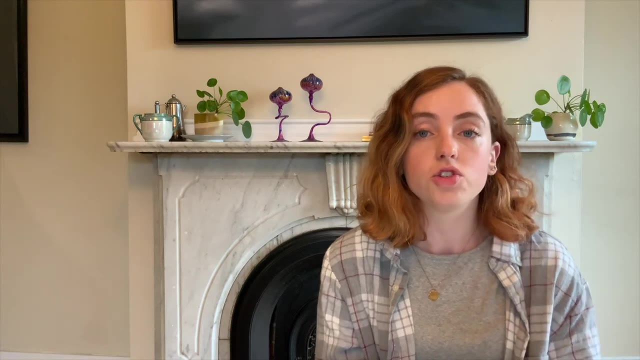 In total, this tells us that he fell approximately 8.45 meters, or 27 meters. So this is the quantity h in our diagram. Now I'm going to estimate the radius of the bridge arch by zooming in a bit on this footage. 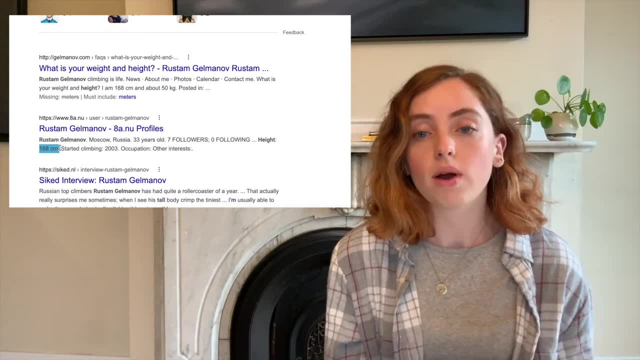 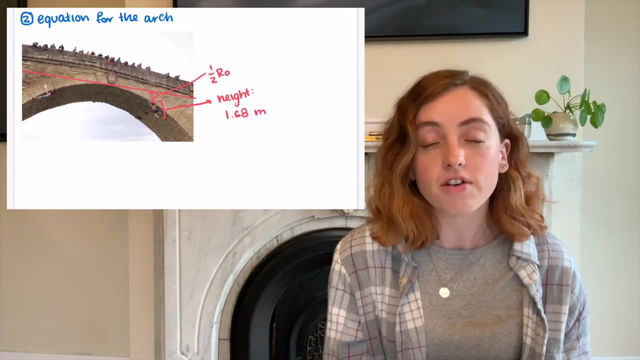 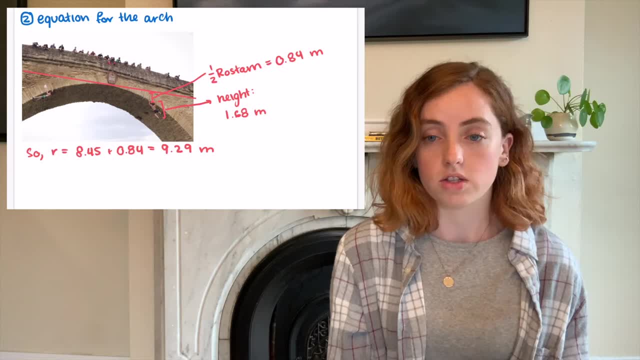 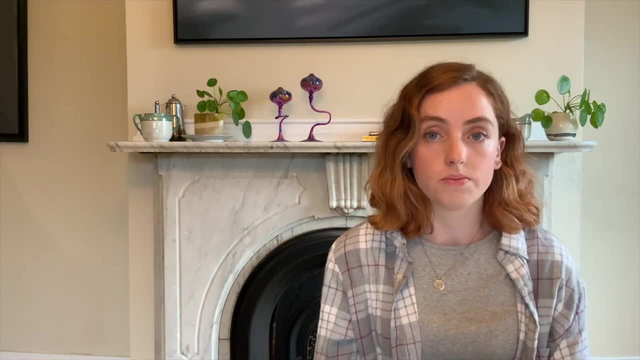 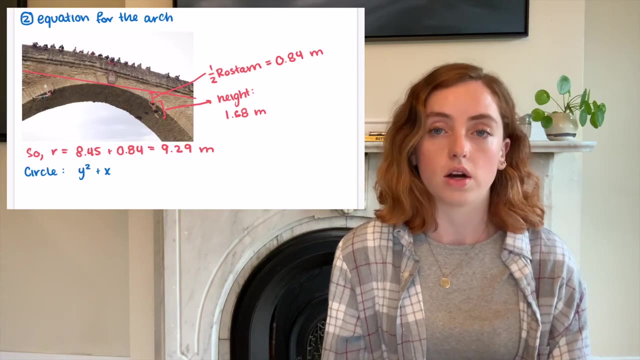 gives us a radius of 9.29 meters, which is approximately 30.5 feet. Now we can write down an equation for the arch of the bridge. I'm going to start with the equation for a circle which is y squared plus x squared equals r squared, where r is the radius We 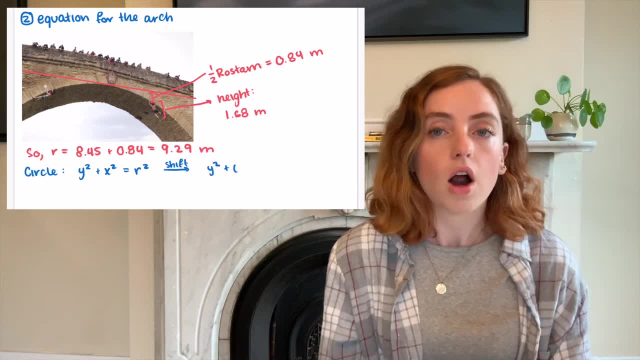 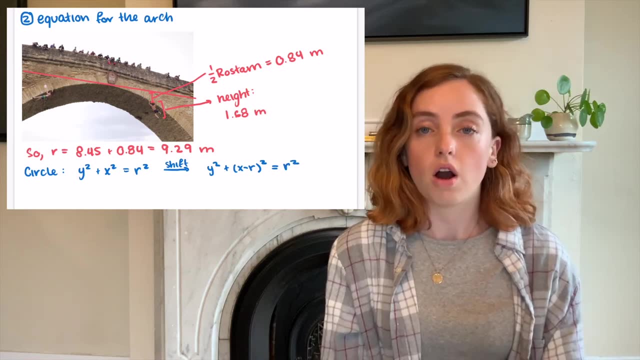 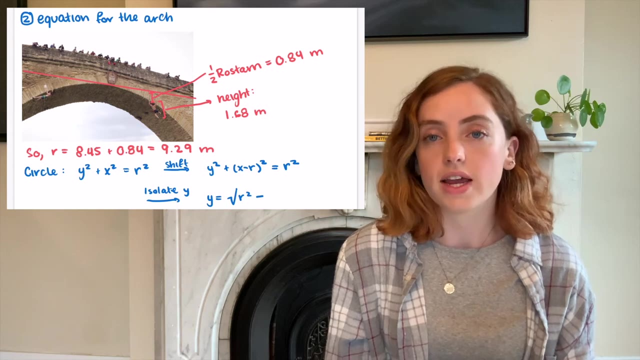 can shift this to the right by subtracting r from x. So we get y squared plus x minus r squared is equal to r squared. From this we'll move the x part to the right side of the formula, isolating y, and then take the square root. In this scenario we want to 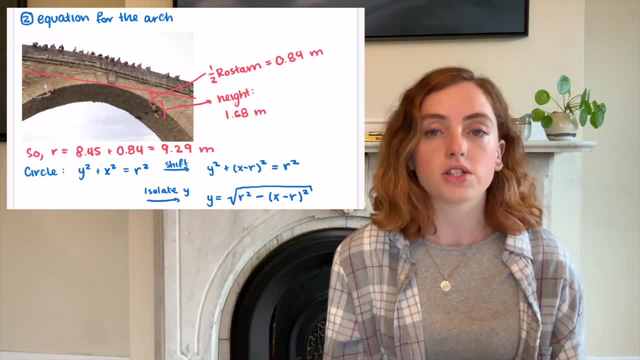 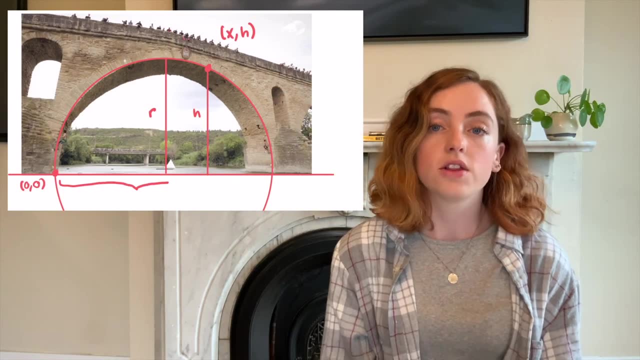 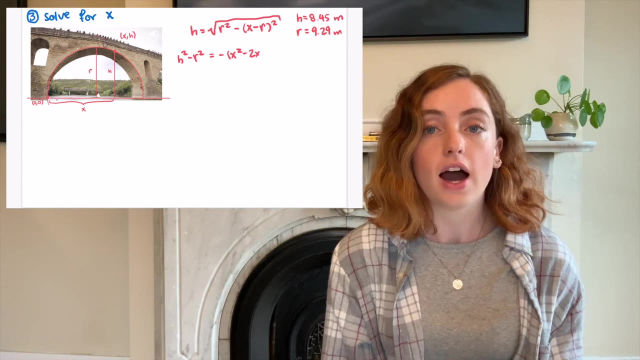 take the positive square root so that we get a semicircle in the upper half plane. This gives us the following bridge equation: Now I want to solve for x the location of Rustam Galmanov when he fell. So I'm going to plug in h for y, since h is the height of the. 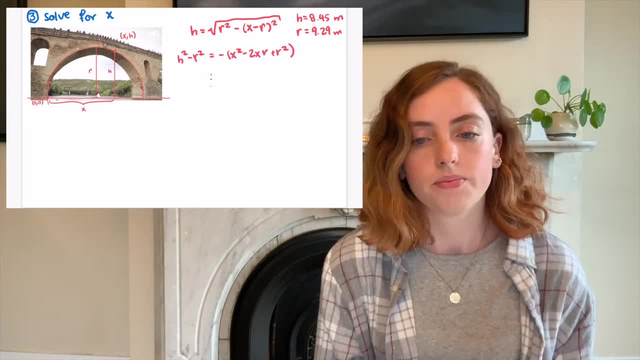 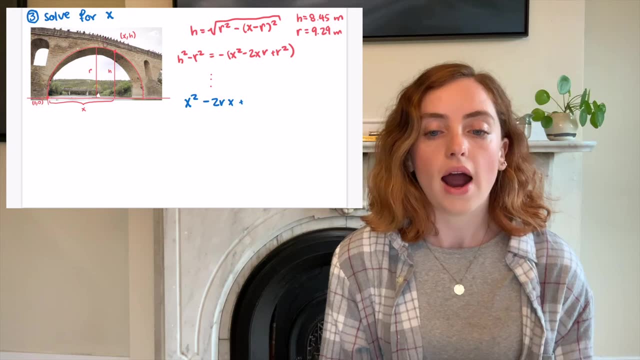 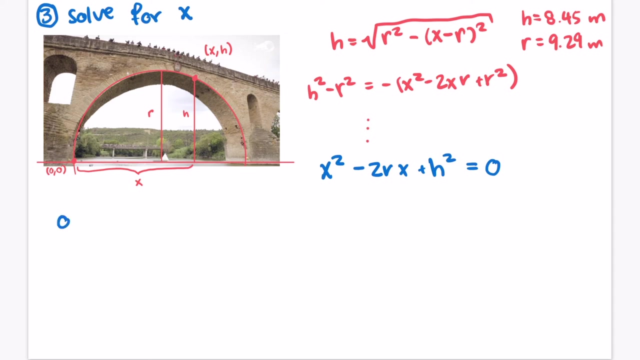 height of his fall, and then I will solve for x. I can rewrite this formula as the following quadratic equation: x squared minus 2rx plus h squared is equal to zero. Now this quadratic formula can be solved using the quadratic equation. The quadratic equation tells us: 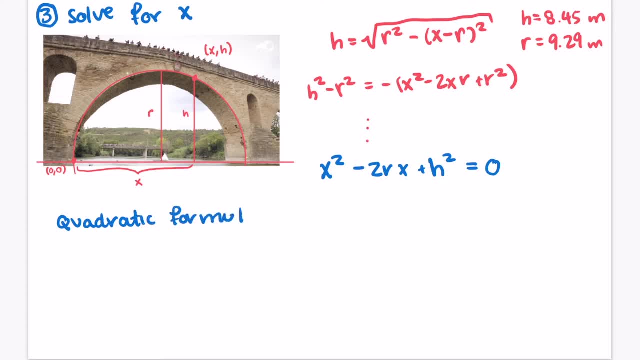 the zeros of a degree two polynomial like this. So this tells us that x is equal to 0.. 2r plus or minus the square root of 4r squared minus 4h squared over 2, which simplifies to r plus or minus r squared minus h squared. We already know the values of r and h from: 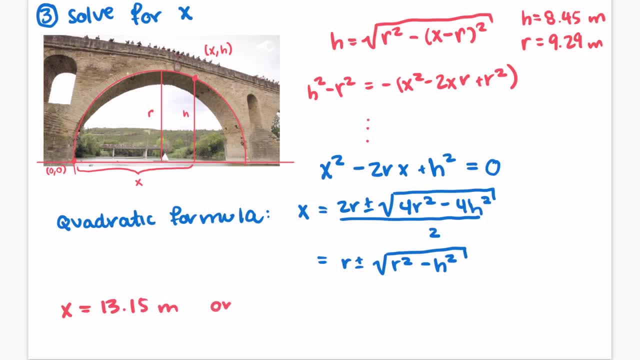 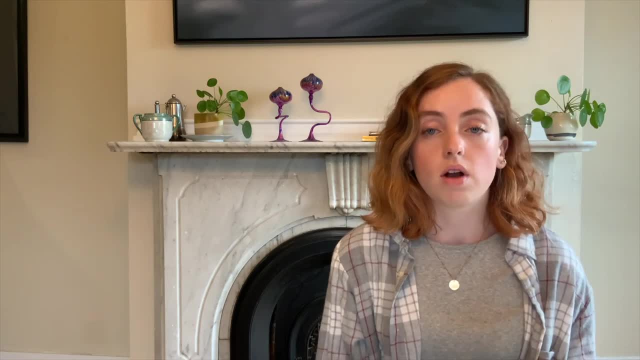 our previous calculations so we can plug those into this formula to get two options for the value of x. This corresponds to the symmetry in the problem. Rustam Galmanov could have started climbing from the left end of the bridge or the right end of the bridge. 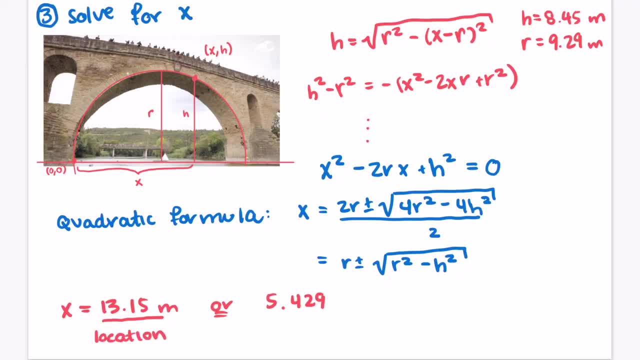 Since he started climbing from the right end of the bridge, we know that his location has to be the greater of the two distances, which is 13.15.. However, this other number, 5.429, actually tells us the horizontal distance that he climbed. This is about 17.8 feet. 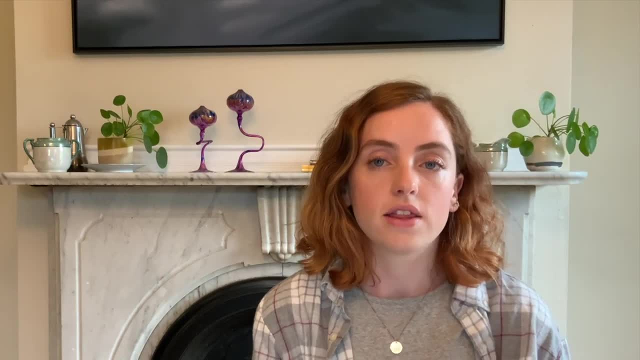 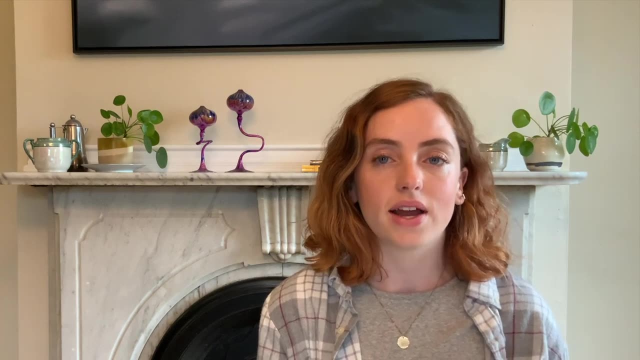 In this video, I use the quadratic formula to analyze the climb of Rustam Galmanov in a 2014 climbing competition. I hope that you enjoyed this video and that you learned something about how to apply quadratic equations to real-life scenarios.